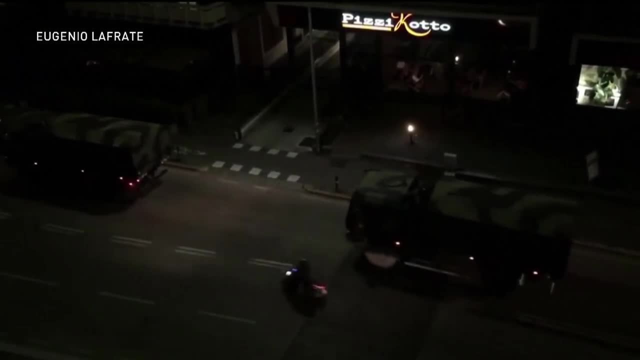 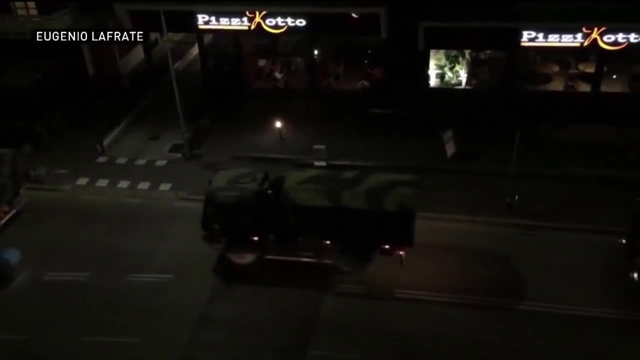 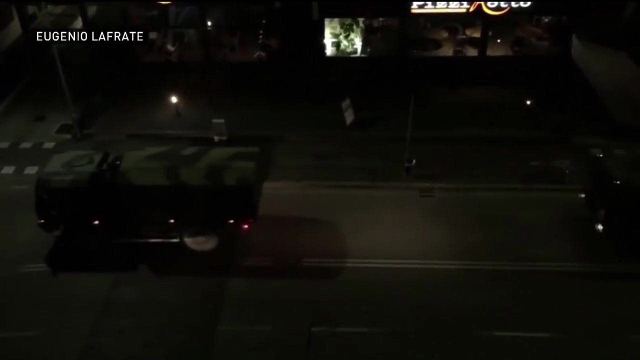 We're getting grim new video out of Italy, where the number of dead as a result of the coronavirus has surpassed China's numbers. We told you this could happen and indeed it did happen overnight. and what you're looking at here- it's dark, but those are military vehicles near Milan: Soldiers. 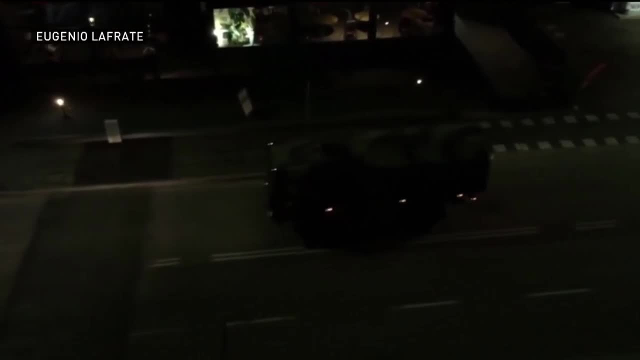 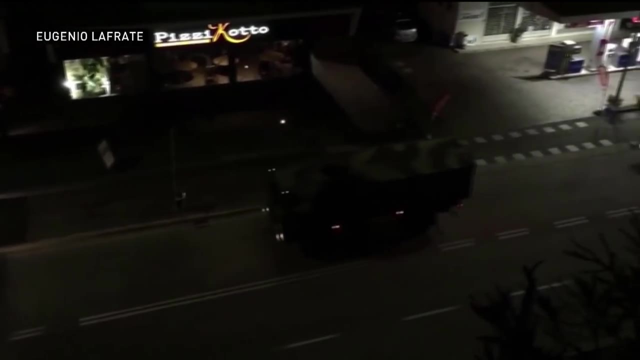 called in overnight to transport the bodies of the dead from Milan to other cities and provinces, because local authorities have been overwhelmed. Funeral homes, cemeteries: there's no more room. Just over 3,400 deaths as of yesterday, a jump of more than 400 from the day before. 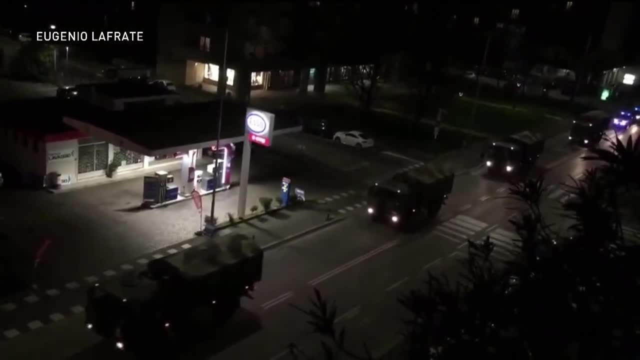 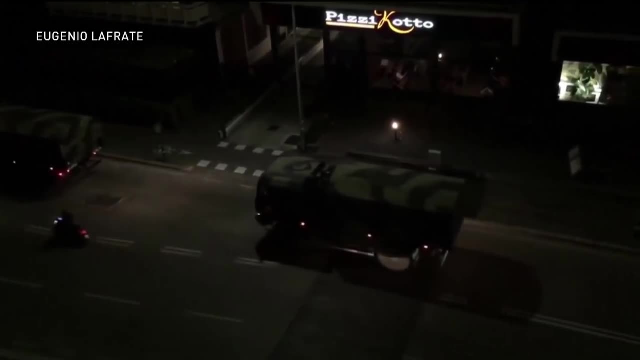 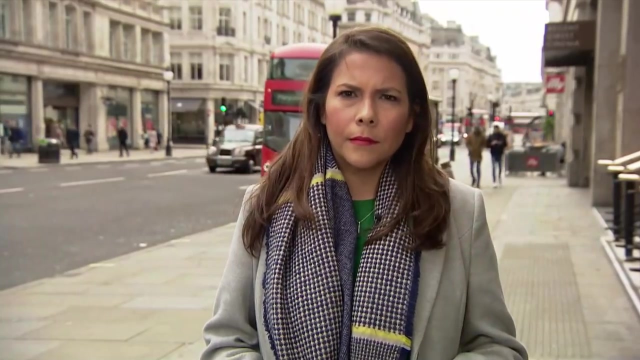 and that, as I said, surpasses China's numbers of dead. Very poignant clip out of Italy: A generation has died. Rene Filippone is tracking the developments in Italy and across Europe and as well the UK picture, and we'll get to that in just a second. but, Rene, I mean, it is just stunning. 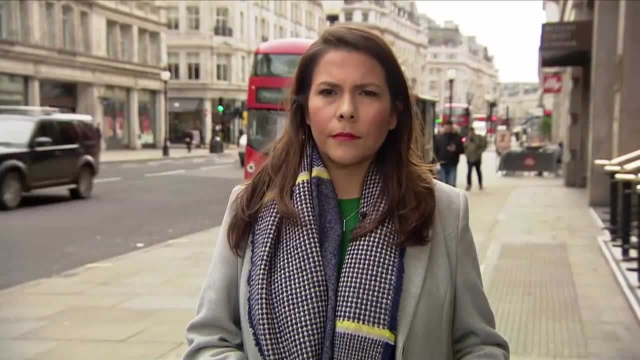 I was reading some comments from the from the area of Bergamo which has seen the greatest number of deaths and funeral director Rene Filippone has seen the greatest number of deaths and funeral directors there. They're burying 600 people when they would normally do about 100. 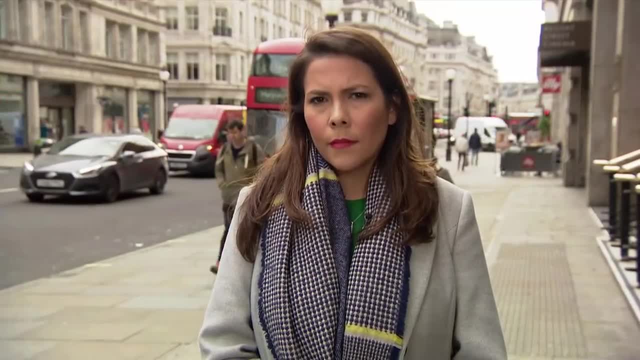 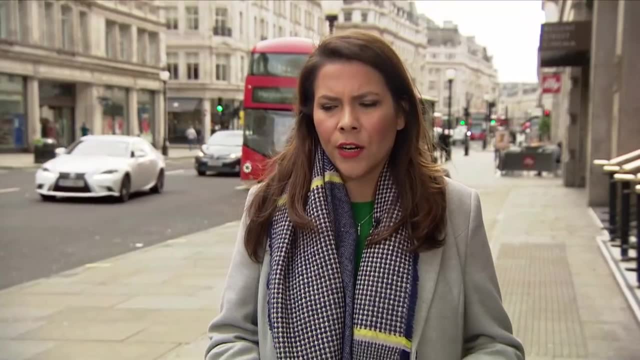 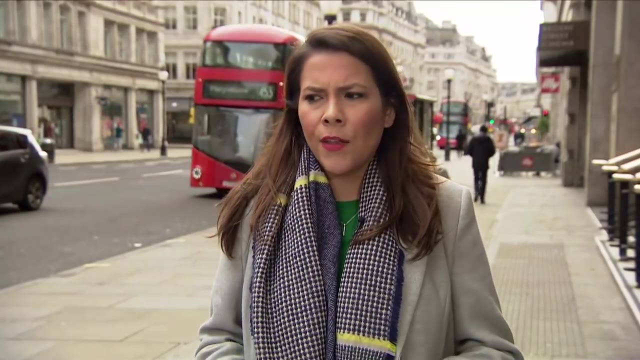 They've never seen anything like it. Yeah, and we're also seeing some video coming out of some of the hospitals in that very hard-hit area and what you see are stretchers with people on ventilators gasping for air. The situation is dire in the hospitals there. We are hearing from doctors on the ground who are saying: you know the? 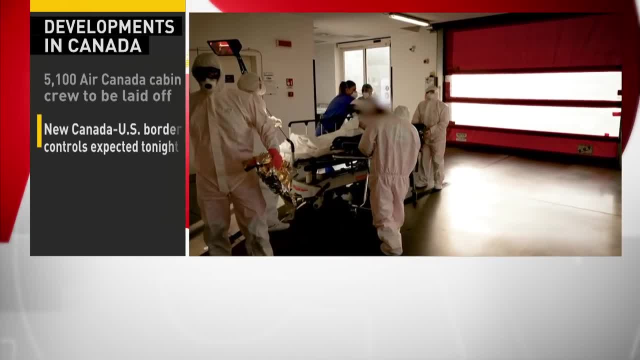 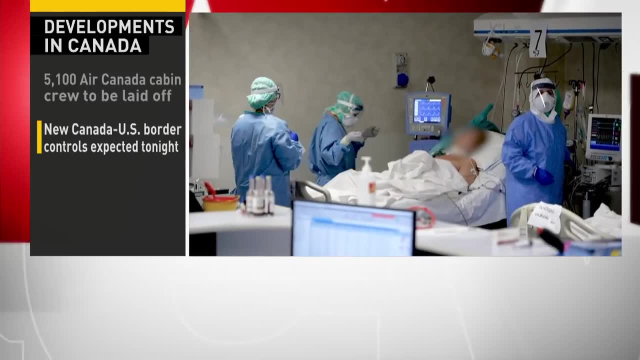 staff are very committed. They're working around the clock, 24 hours a day, coming in when it's not even there And they're just stuck in that same familiar shift. but they just can't keep up. One of the men who heads up the ICU says the hospitals, they're at a breaking point, They are running out of equipment. 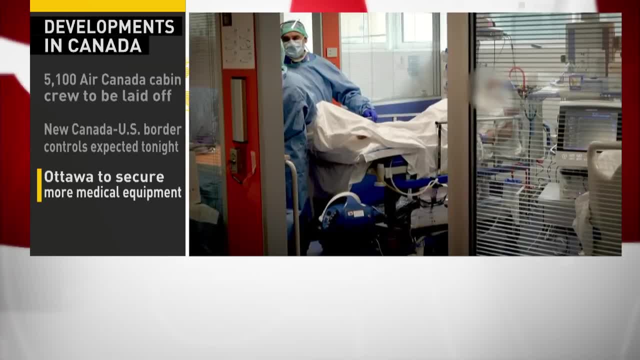 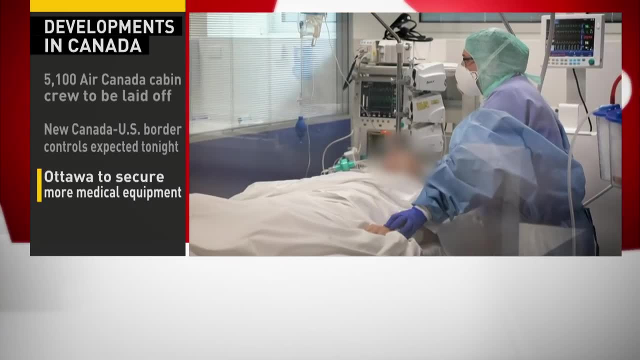 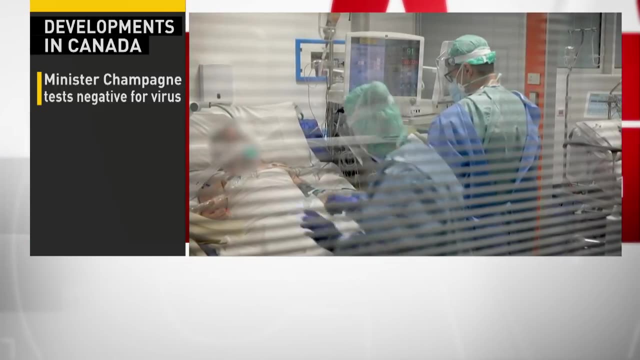 gear space and, most importantly, workers. And a big problem here in Italy specifically is that 8% of the positive COVID-19 cases are doctors, nurses, healthcare workers. In fact, more than a dozen doctors have died Now. one of the ways they're trying to relieve some of that pressure is they're bringing in a cruise ship, one off the coast of Germany, and another one they're bringing in is a cruise ship one off the coast of Germany. One of the ways they're trying to relieve some of that pressure is they're bringing in a cruise ship, one off the coast of Germany.